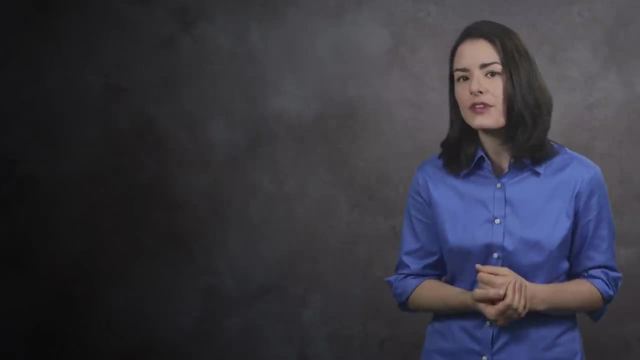 By adding features we're familiar with from the real and complex numbers, we'll arrive at the full definition of a field. 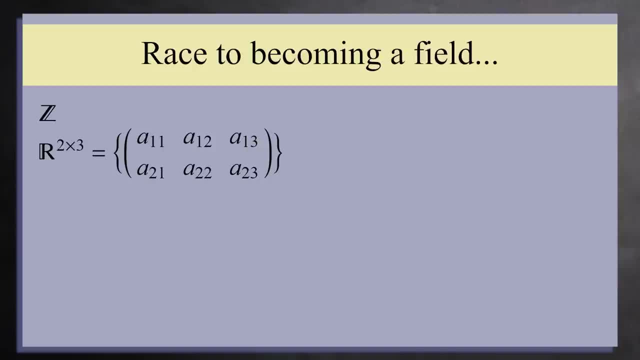 Consider these six sets. The integers. The 2x3 real matrices. The 2x2 real matrices. The rational numbers. The integers mod 5. And the integers mod 6. 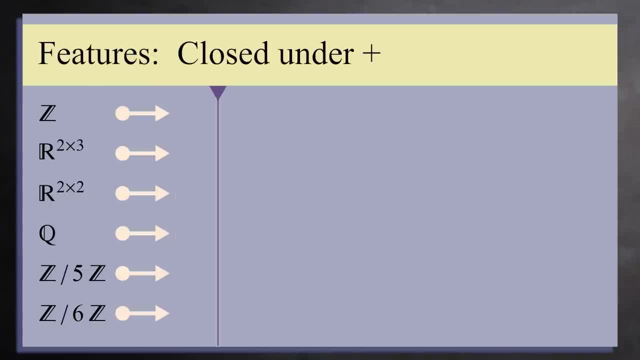 Notice that all six sets are groups under addition. They're closed under addition. You can add any two elements together and the sum is in the set. The negative of each element is in the set. There's an additive identity and the associative property holds. Better still, all six groups are commutative under addition. So as a first pass, all six objects are commutative groups under addition. The next feature we'd like to include is multiplication. 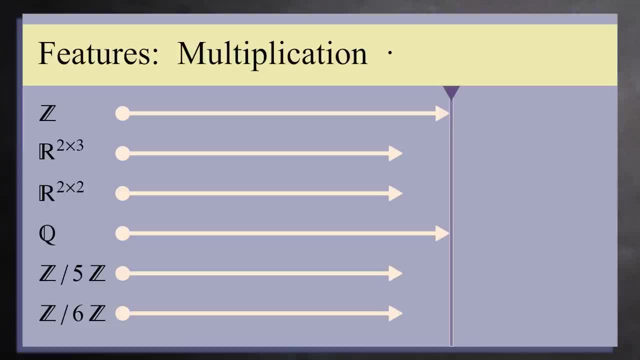 You can multiply any two integers or rational numbers together. 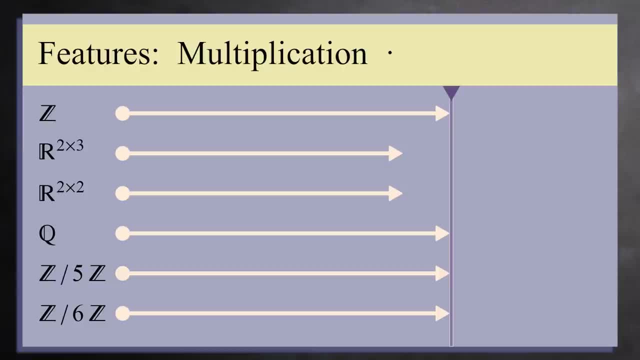 You can also multiply any two numbers mod n for any n. That leaves the two sets of matrices. You can multiply two square matrices, but you cannot multiply 2x3 matrices by each other. Their dimensions are incompatible for multiplication. 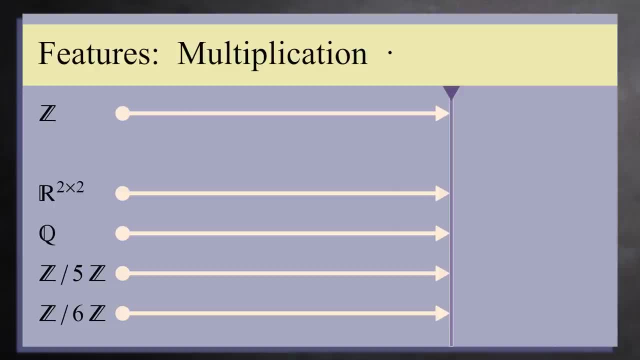 So only five of the six sets advance to the next round of commutative groups with multiplication. Just like the first set, you can also multiply any two numbers mod n for any n. 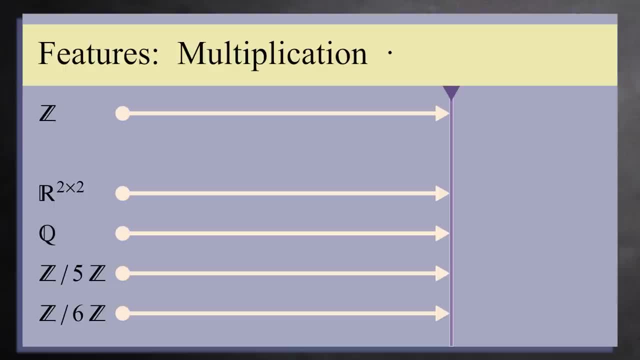 Just as all the groups are commutative under addition, in the field, we'd like multiplication to be commutative as well. After all, the real and complex numbers are both commutative and they are a pleasure to work with. 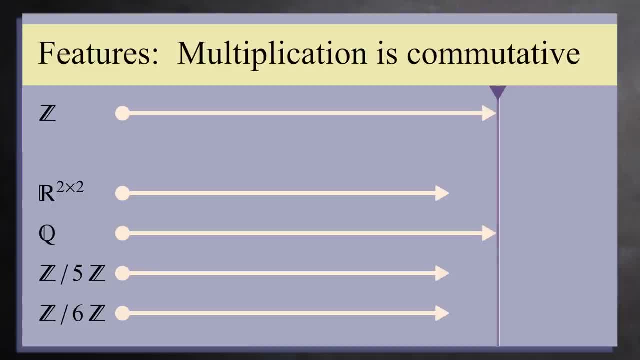 The integers and rational numbers are both commutative under multiplication, so they advance. 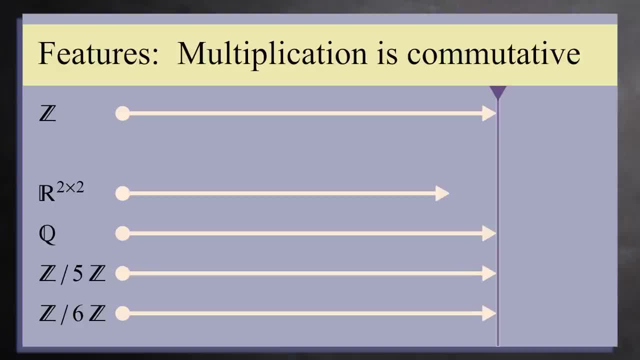 Also, the integers mod n are commutative under multiplication for any n. But we're about to lose another candidate. The 2x2 matrices are not commutative under multiplication. They're commutative under multiplication. 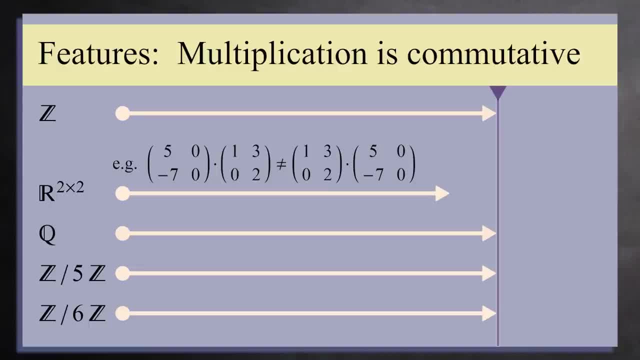 There are an infinite number of examples where matrix multiplication is not commutative. Here's one example. 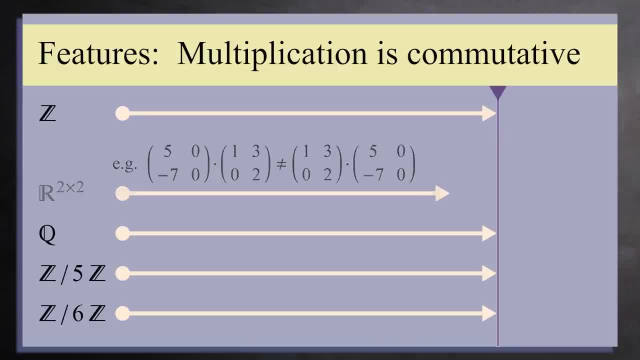 So only four of the six are commutative under multiplication. 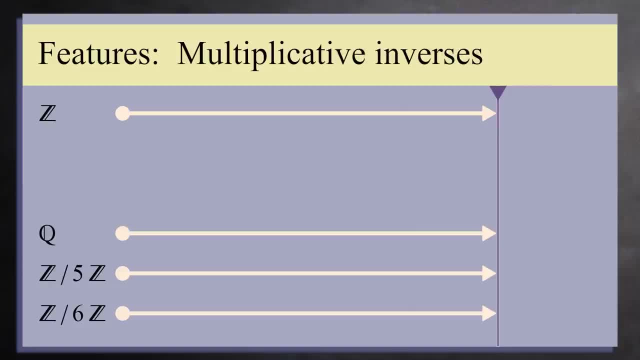 Next, we'd like each number to have a multiplicative inverse. The additive inverse 0 is a big exception here. 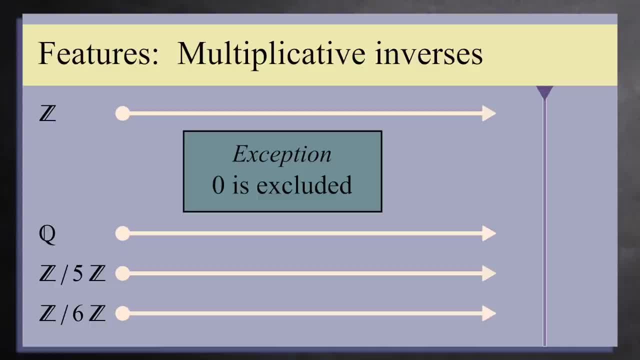 You cannot divide by 0, so this number cannot have a multiplicative inverse. 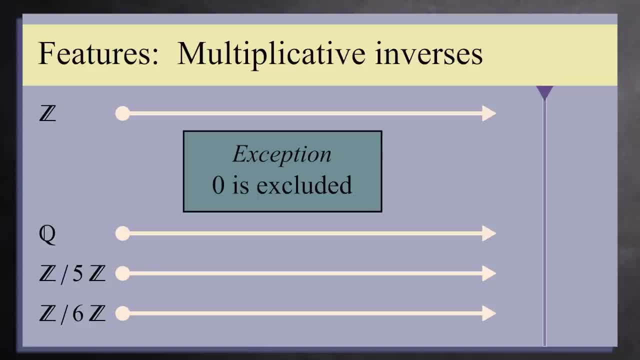 But we'd like every non-zero number to have a multiplicative inverse. Sadly, we're about to lose two more. So we're going to multiply by 2x2. 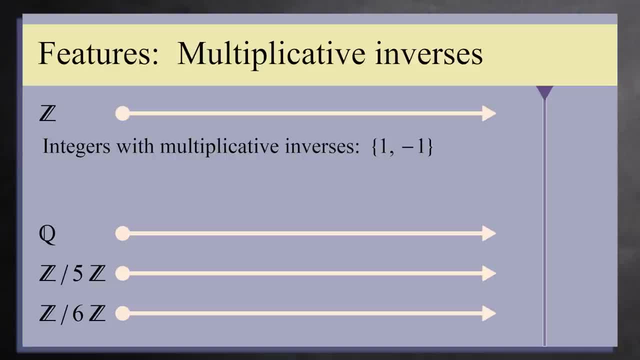 In the set of integers, only 1 and negative 1 have multiplicative inverses. 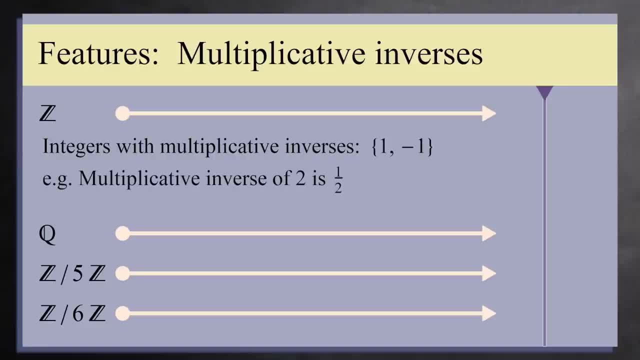 None of the other integers have one. For example, the inverse of 2 under multiplication is ½, which is not an integer. And we lose the integers mod 6 as well. 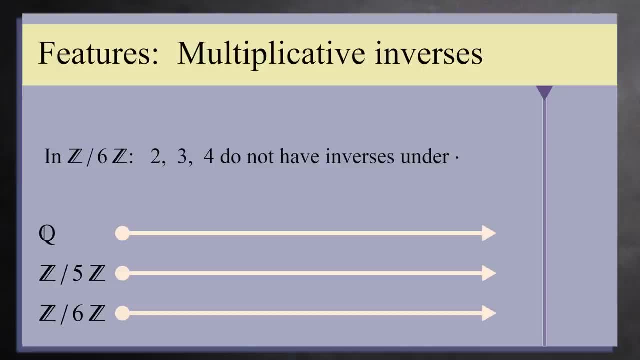 2, 3, and 4 do not have inverses mod 6. 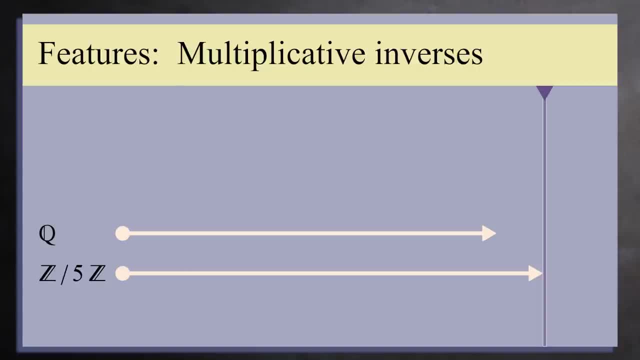 Mod 5, however, is different. Here, every non-zero number has a multiplicative inverse. You can check this by looking at the multiplication table for the set. this set. 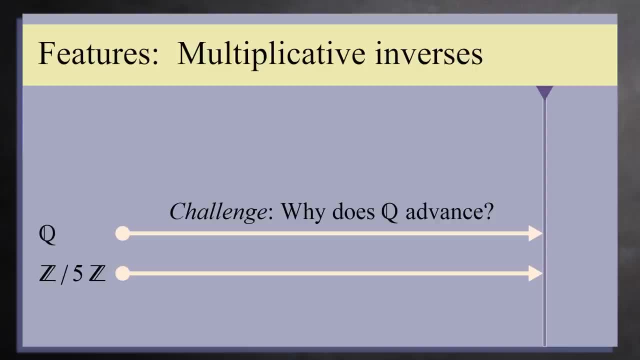 So the only two sets to advance are the rational numbers and the integers mod 5. 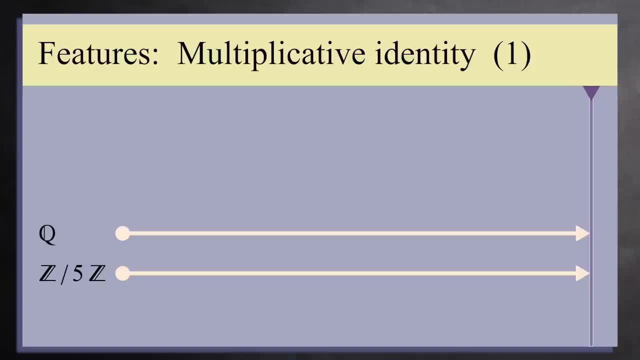 By the way, these two sets both have a multiplicative identity 1. This is not a surprise, since the product of a number and its multiplicative inverse is 1. 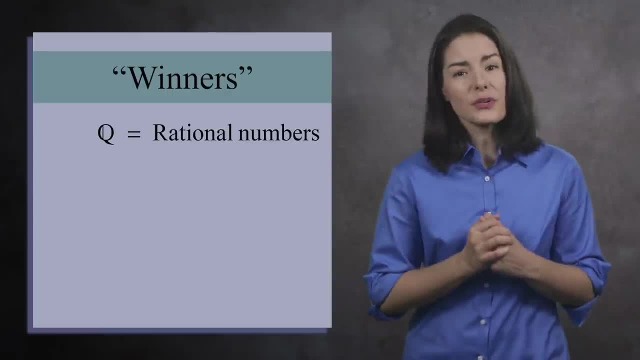 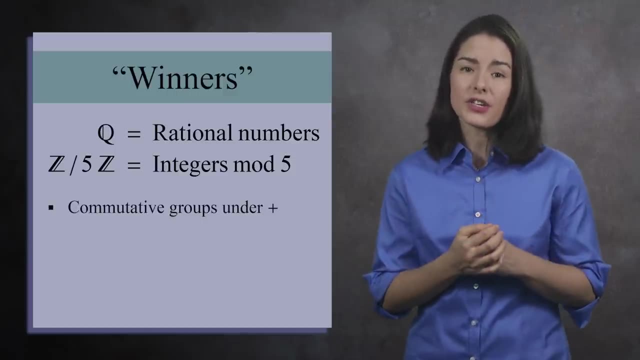 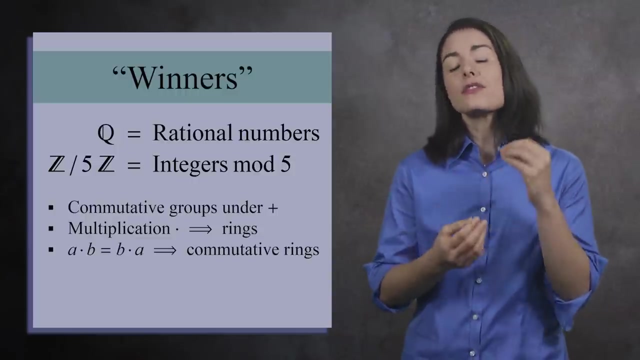 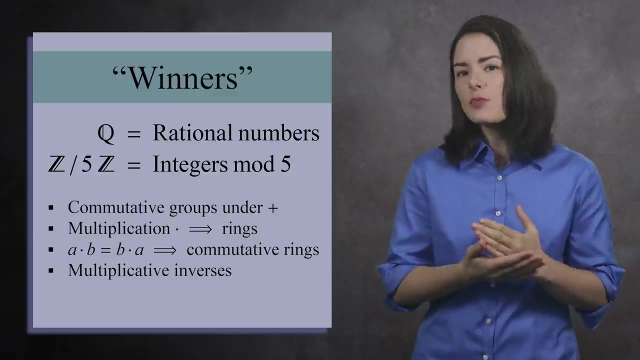 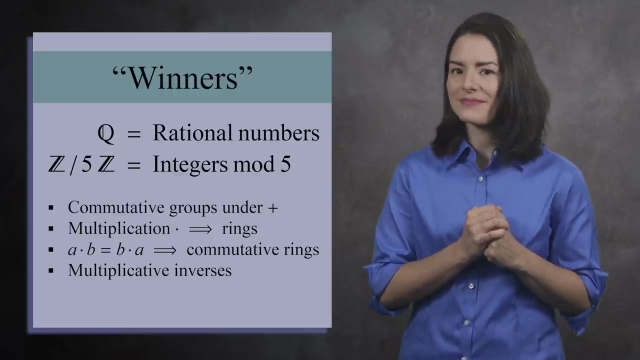 The race is over, and we have two winners! The rational numbers and the integers mod 5. These both share a similar set of properties. They are both commutative groups under addition. They both have a second operation, multiplication, which makes them rings. Furthermore, multiplication is commutative, so they are commutative rings. Better still, other than 0, every number has a multiplicative inverse. It's this last property which puts them over the top and turns them into fields. We're now ready for the textbook definition of a field. 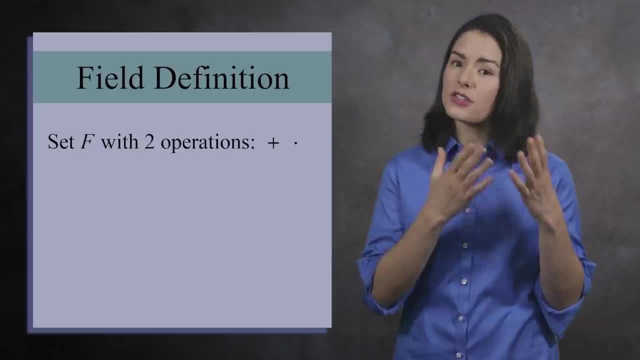 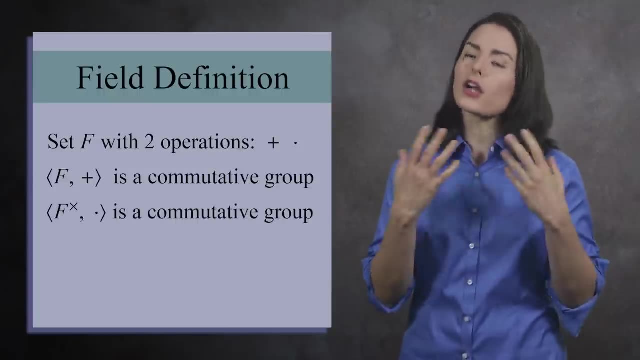 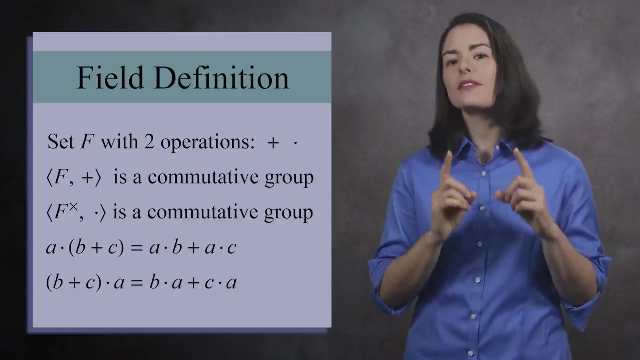 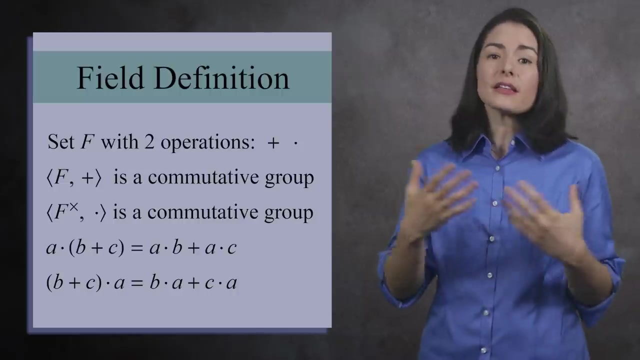 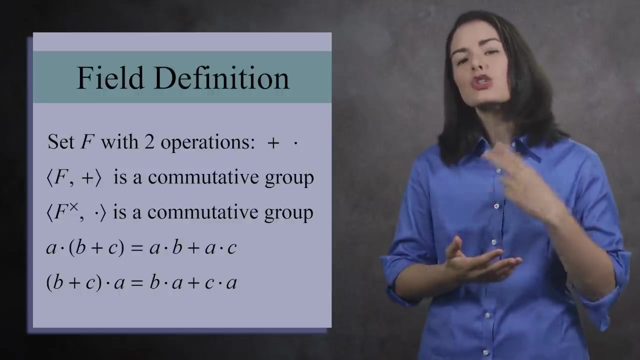 A field is a set of elements f with two operations, addition and multiplication. Under addition, the elements are a commutative group. Under multiplication, the non-zero elements are a commutative group. Also, addition and multiplication are linked by the distributive property. This is the compact definition of a field. If you wanted, you could define a field and make no mention of groups whatsoever. You could just give a complete list of all the properties a field must satisfy. This is fine. But you do lose sight of the fact that a field is actually two groups with two operations at the same time. Let's return to the two examples of a field we just looked at. Let's return to the two examples of a field we just looked at. Let's return to the two examples of a field we just looked at. 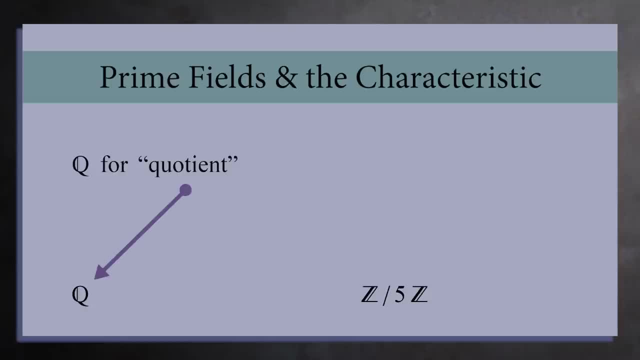 The rational numbers and the integers mod 5. The rational numbers are denoted by q for quotient, since every number in this field is a quotient of two integers. The rationals are an infinite field, while the integers mod 5 are a finite field. 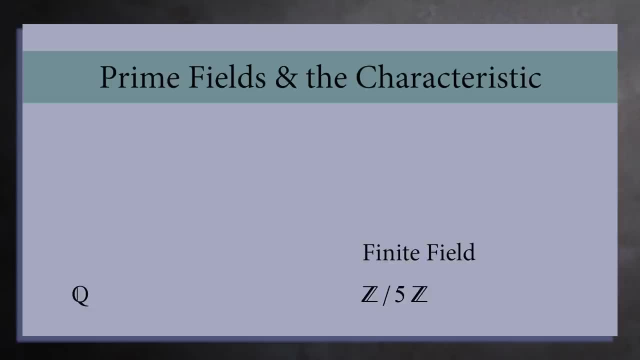 But the integers mod 5 are not the only finite field. In fact, the integers mod p for any prime number p is also a field. 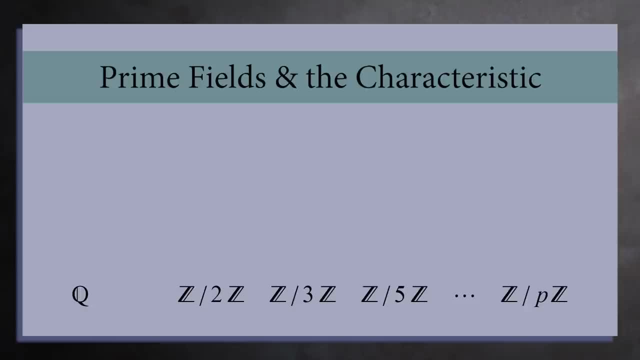 Together, these form the starting points for all fields. That is, if you pick any of the following fields, the integers mod p for any prime number p is also a field. any field f, then it will contain one and only one of these fields as a subfield. 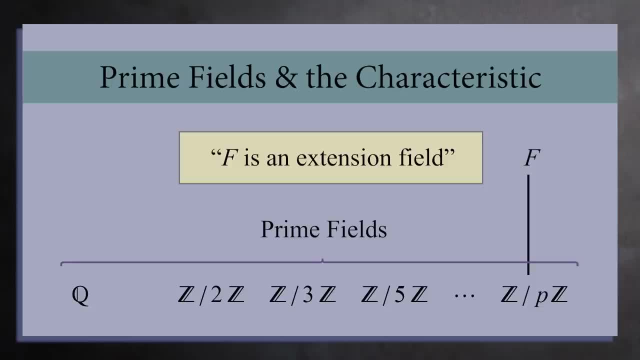 We call these fields prime fields, and say that f is an extension field. If f is an extension of the integers mod 2, we say it has characteristic 2. If it's an extension of the integers mod 3, it has characteristic 3. And if it's an extension of the integers mod p, we say f has characteristic p. But if f is an extension of the rational numbers, we say it has characteristic 0. 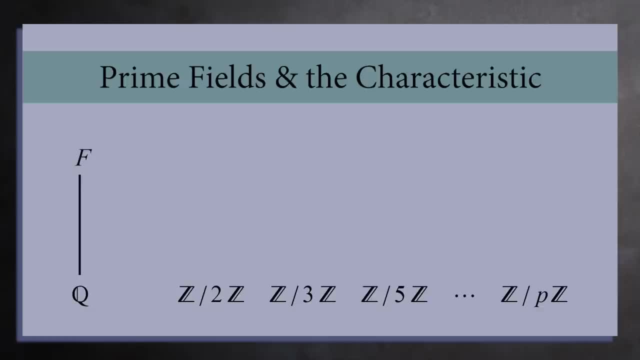 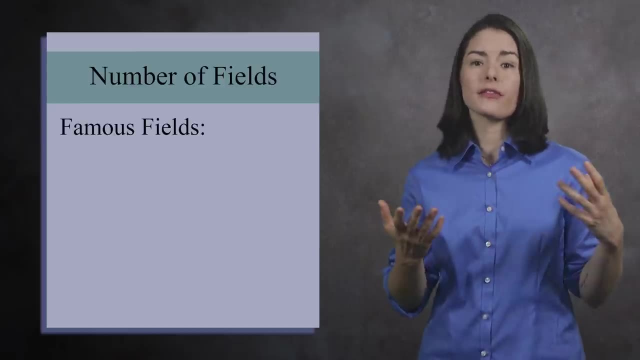 So the characteristic of a field tells us which prime field it extends. There are an infinite number of fields in mathematics. We begin by learning about the big three, the rational numbers, the real numbers, and the complex numbers.